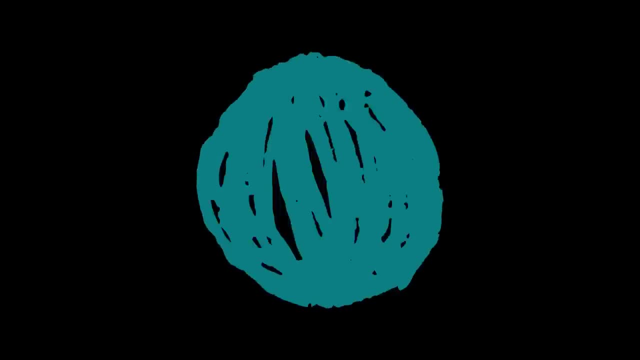 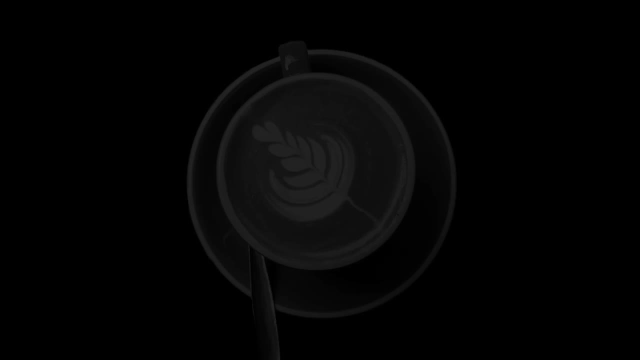 Let's say, your close friend Lee confides in you that they're struggling with depression. They're feeling isolated and alone, But whenever they're invited to go out they find it impossible to do. Lee insists they don't want anyone else to know. They're trusting this information. 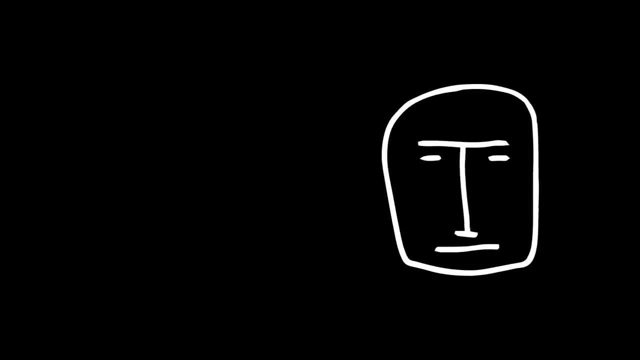 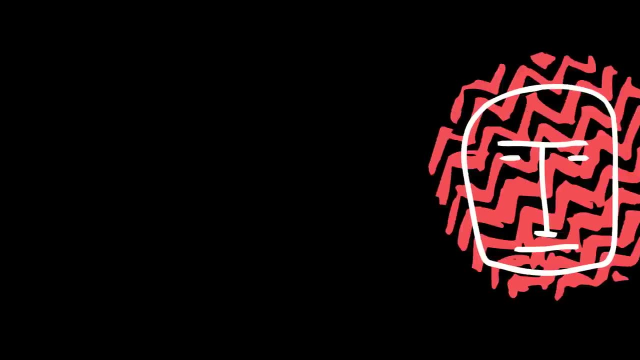 to you alone. A few days later, another friend comes to you asking you to help them out. Lee says he hasn't had a chance and he's been trying and trying to make better plans. Lee's flaked on plans at the last minute yet again, And your friend has had enough. 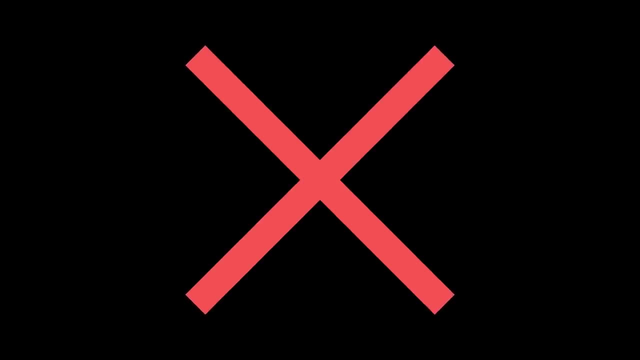 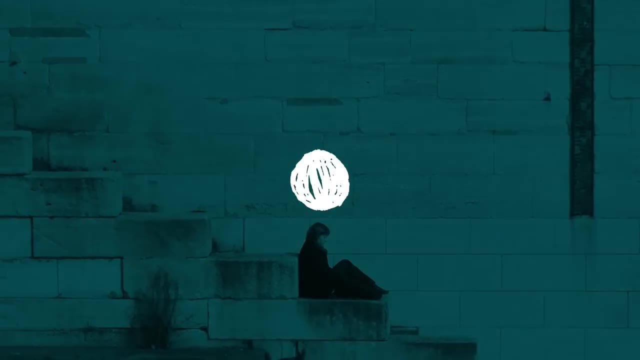 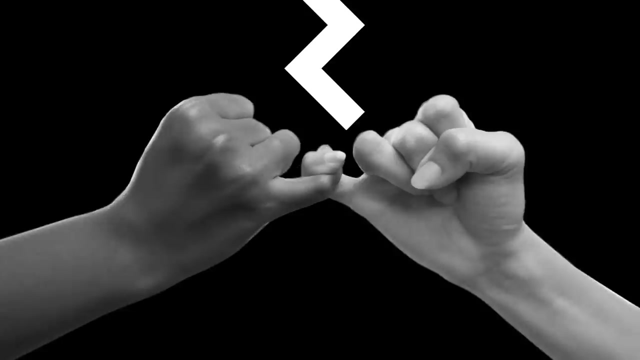 They've decided they just won't bother inviting Lee out anymore. so you're torn. If Lee stops being invited to things, the isolation could make them feel even worse. Sharing information about their depression might help Lee be treated with more empathy and compassion, But it would be a breach of trust. And if Lee found out, especially in 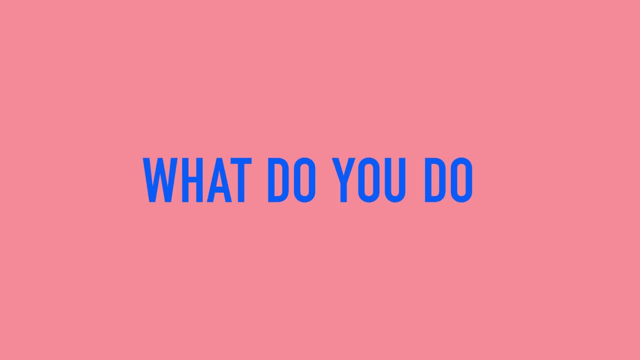 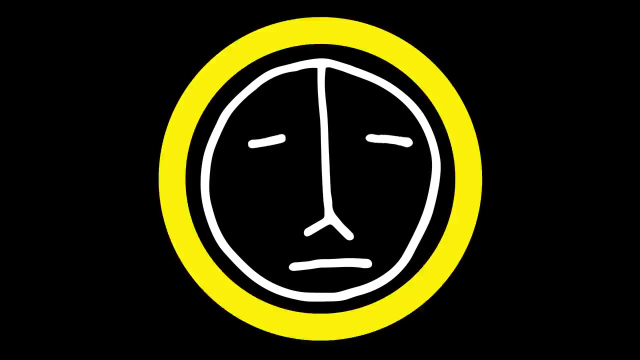 a vulnerable state. who knows what he's going to do knows what might happen. What do you do? Keep the secret and allow Lee to be socially isolated, Or break Lee's trust, but do it for their benefit. Answering this question means getting clear on what matters, Our values and principles. 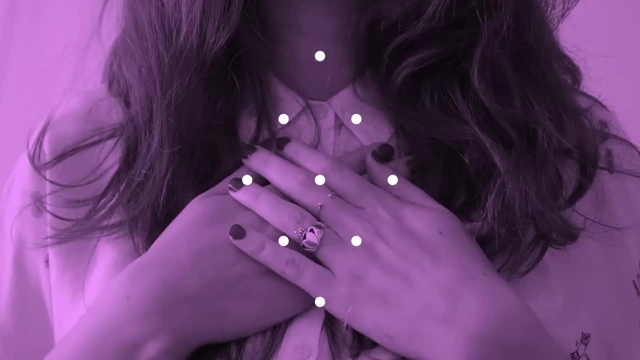 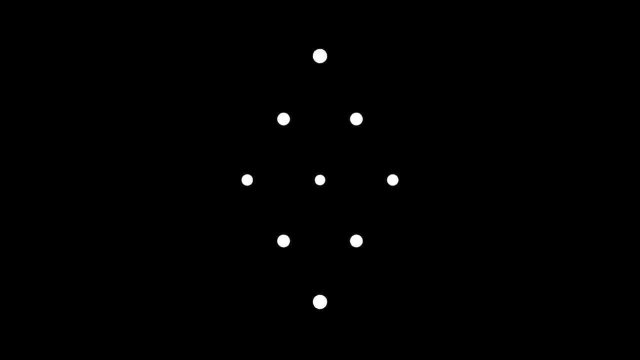 Our values are the things we hold to be good and therefore care about most deeply, Things like justice, knowledge, family and equality. In this case, we're likely to value both the trustworthiness and compassion which pull us in different directions. So it looks like an appeal to values alone. won't let us. 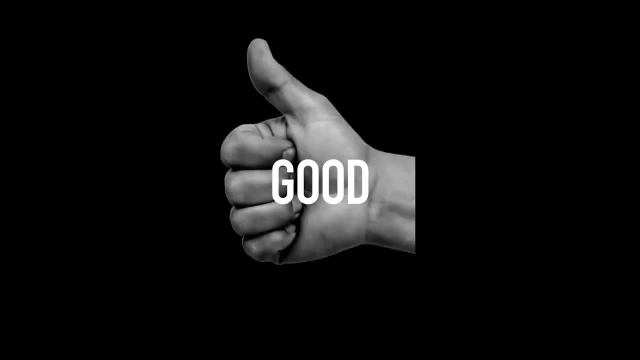 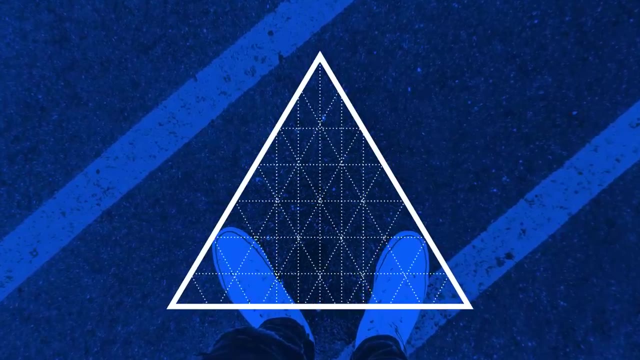 solve this dilemma. We don't just need to know what's good, we need to know what's right. This is where principles come in. They help us draw a line in the sand. They determine the acceptable ways of getting the things that we value. So 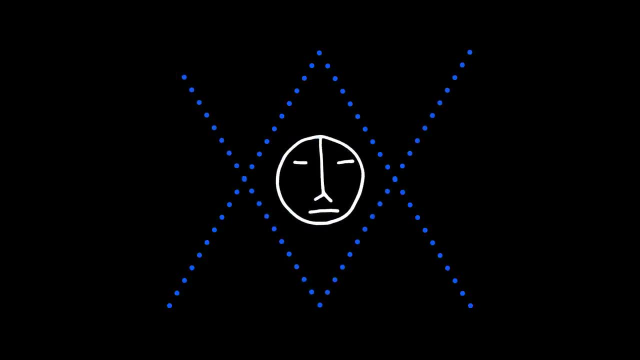 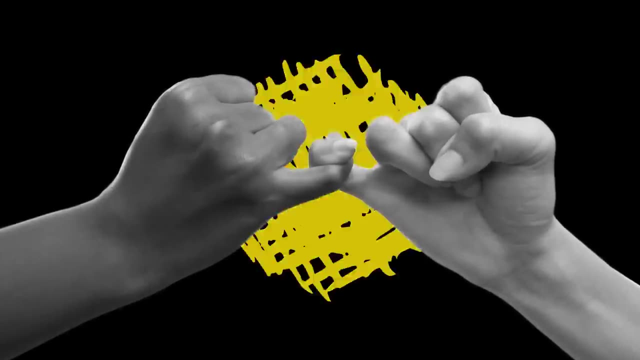 what's our guiding principle with regard to Lee? Some people think that it's important for us to be honest with ourselves and not be selfish. Some people might adopt a principle like be true to your word, meaning you keep Lee's confidence no matter the risks Others might be. 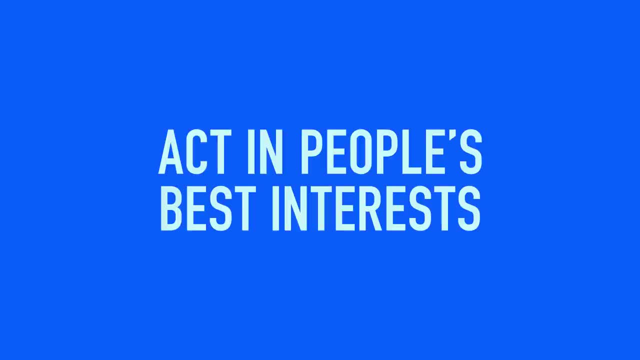 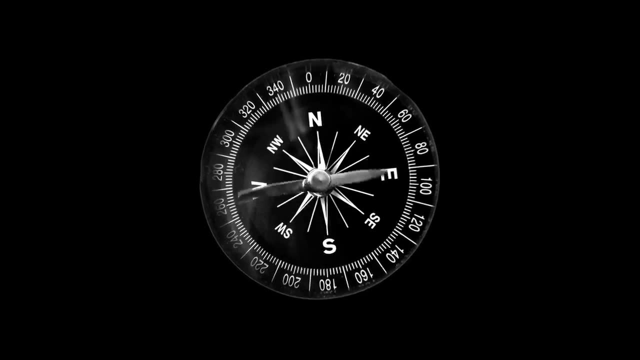 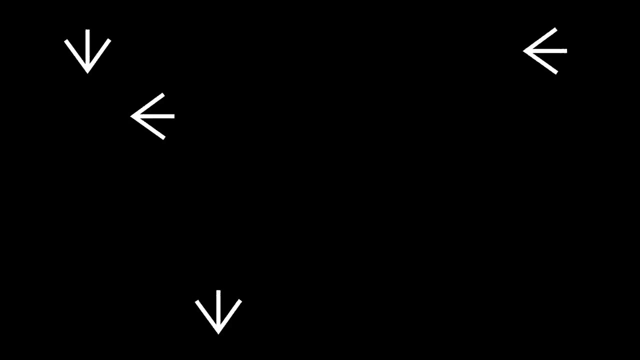 inclined towards a principle like: act in people's best interests and decide that it's in Lee's best interest that people know about the depression. Of course, there are still ambiguities, which is part of what makes ethical decision making so complicated. So how do we select which values and principles to